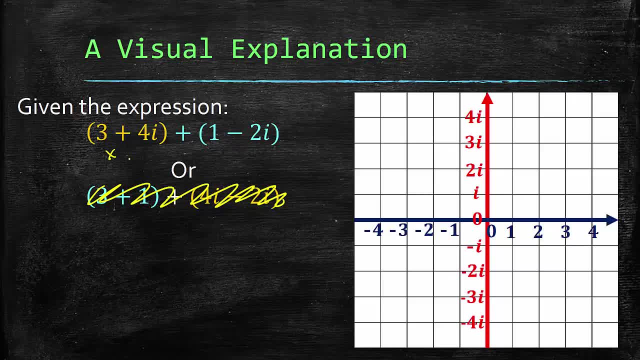 If I gave you this right here, you could think of this as like an x coordinate and a y coordinate, So we'd have three and then four i, which would be right there, And then we would be adding one minus two i. So you add your constants together and your imaginary numbers together. 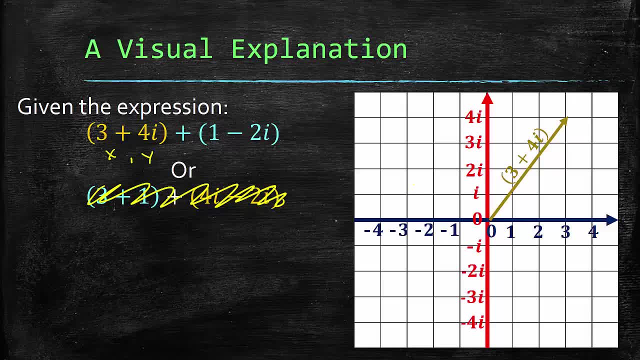 So three plus one is four, So we'd be going further to the right, And then we'd be subtracting two- i, so we'd be going down, And that would be kind of our new spot of four plus two i, Or so that's just a visual representation. 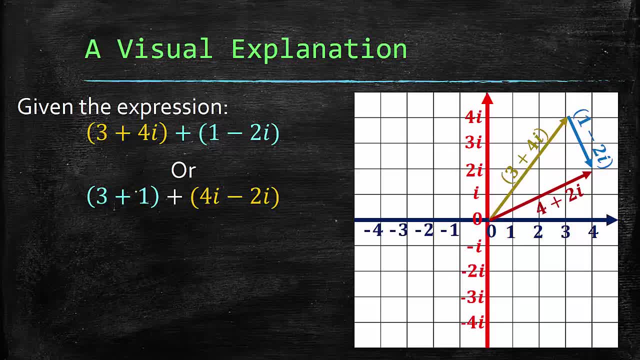 This is a more traditional way of doing it. I would suggest grouping your numbers, So you have your constants and then you have your imaginary numbers. Don't forget the sign to the left of it. Put them together: three plus one is four. four i minus two i is just two i. 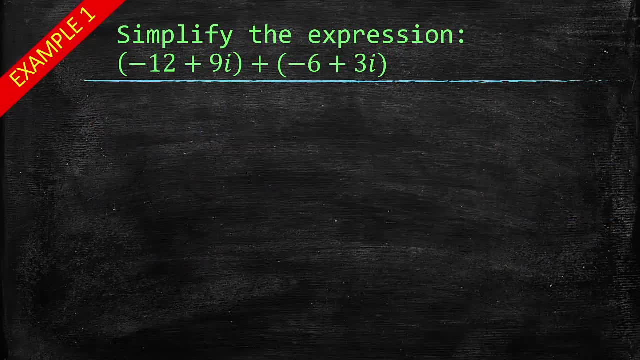 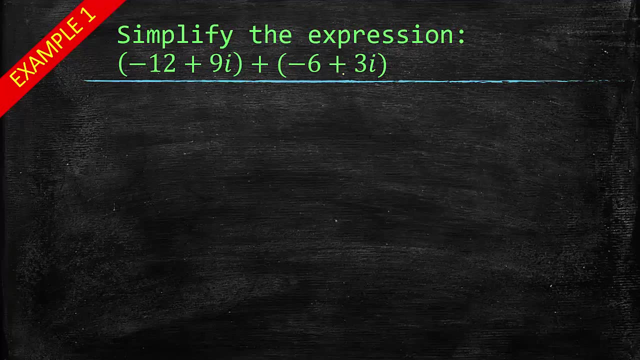 All right. so simplify the following expression: We have nine, We have negative 12 plus nine i plus the quantity negative six plus three i. So this is just addition or subtraction. We have this in between, which means realistically we can, we don't have to worry too much about. 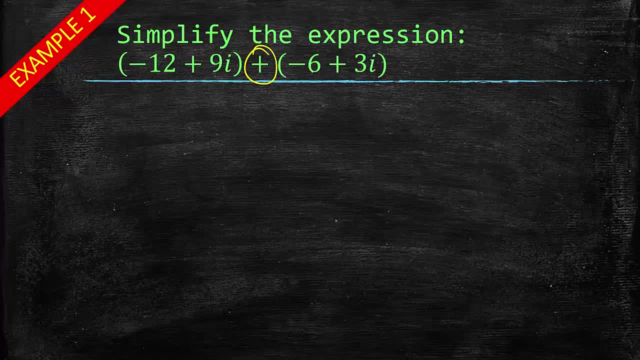 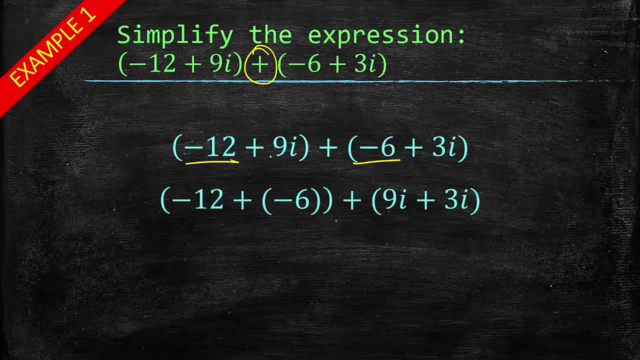 the parentheses. It's a positive. So really we can just get rid of the parentheses if we want to. But again, I would suggest grouping: So negative 12 plus negative six, and then nine, i plus three, i Okay. So negative 12 and negative six. 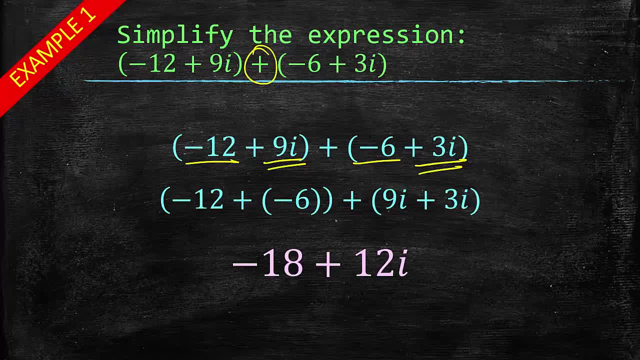 Negative six, because it's negative 18, nine i plus three i 12. i. So notice we're treating this just like we would a variable, as if it were like nine x plus three x, That'd be 12 x, right. 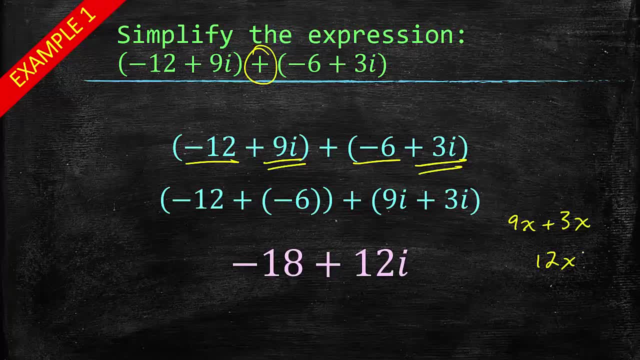 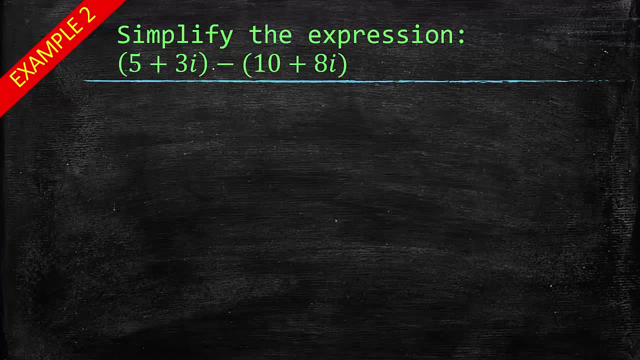 Same thing. The trick comes when we start getting the powers of that. All right again. simplified expression. This is addition or subtraction, So now we just can't remove the parentheses. We actually have to distribute this negative sign to both terms inside. 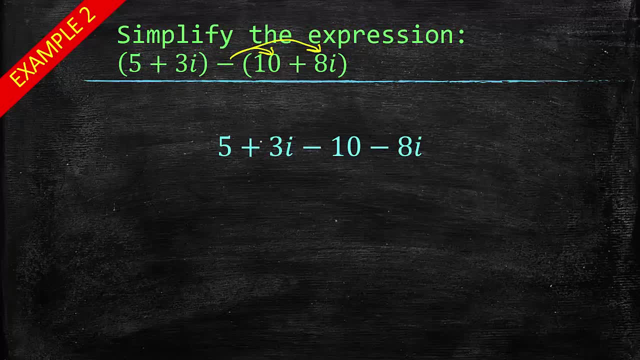 All right, So we do that It's going to become. we've still got the five plus three out in front, but this negative side becomes negative 10 minus eight i. So now we can lose the parentheses Again. take the numbers and the sign to the left of them. 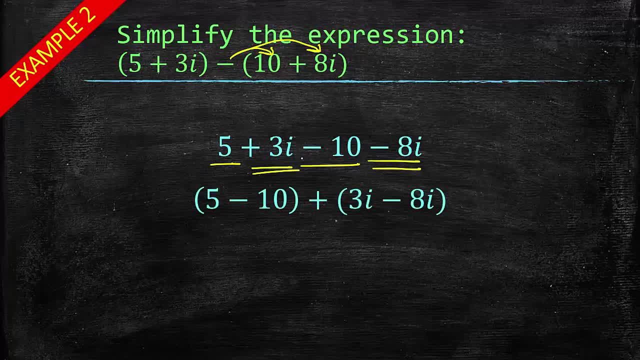 Okay, So we have a five and a negative 10 and three i minus eight i. Five minus 10 is negative five. Three i minus eight i is negative five i. So we have negative five minus five i for your answer, All right. 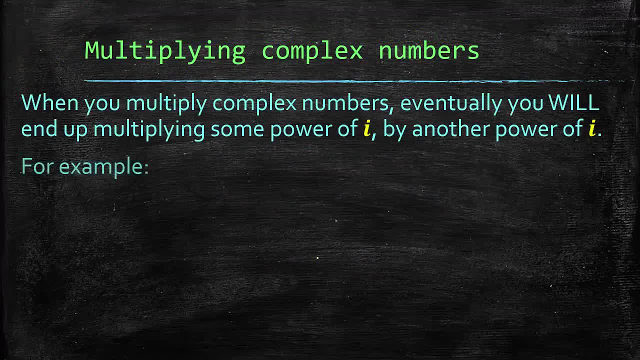 All right, All right. Now, when you're multiplying complex numbers, eventually you will end up multiplying by the power of i- Okay, Some power of i. by another power of i. For example, if you had i times i, that would be i squared right. 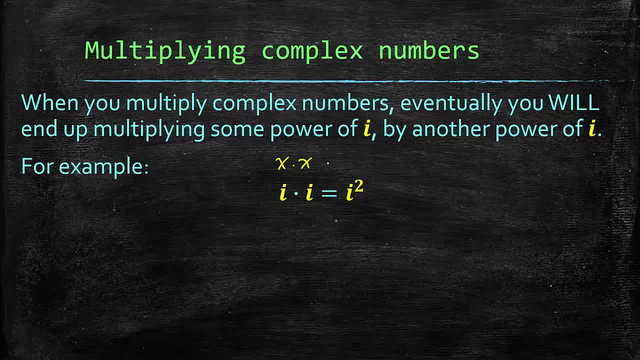 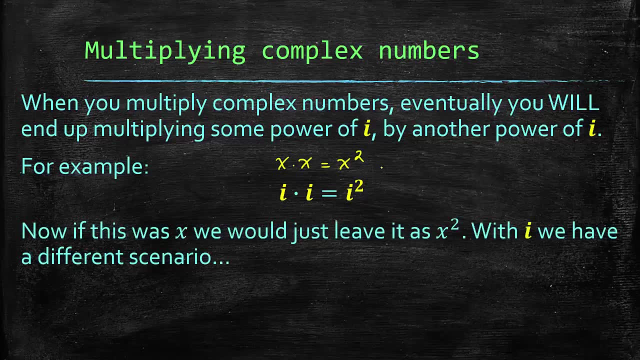 Because I said we're treating this like as if we had variables and x times x is x squared. So yes, that's absolutely true. However, unlike as if it were x squared, where we would just leave it as x squared with i, we have kind of a different scenario once we get into the powers of i. 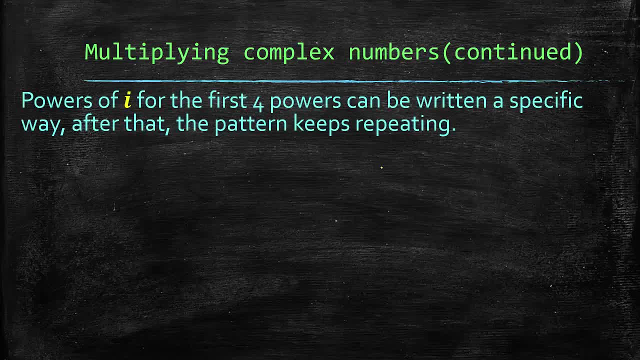 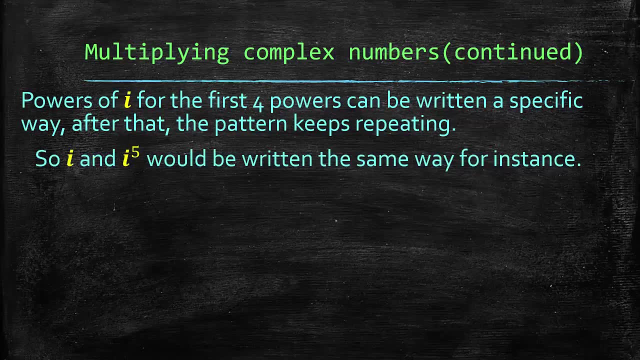 All right. So let's look at this. Okay, The first four powers can be written a specific way, and after that the pattern keeps repeating. So, for example, i and i to the fifth, or we could say i to the first. okay, because they're. 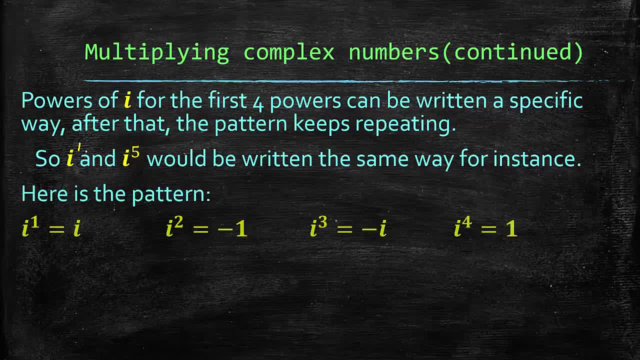 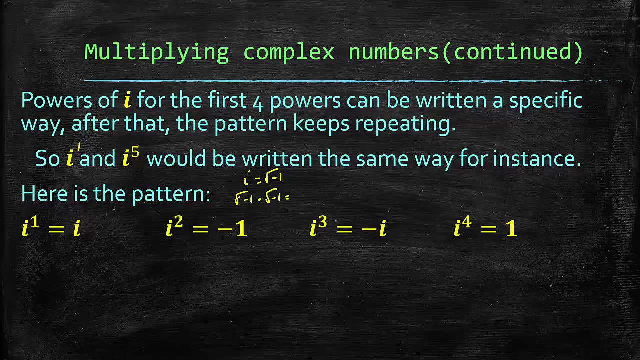 the same thing would be written the same way. So here's the pattern: i to the first power, that's just i. i squared is negative one Because, remember I said that i is the square root of negative one. So if you have the square root of negative one times the square root of negative one, 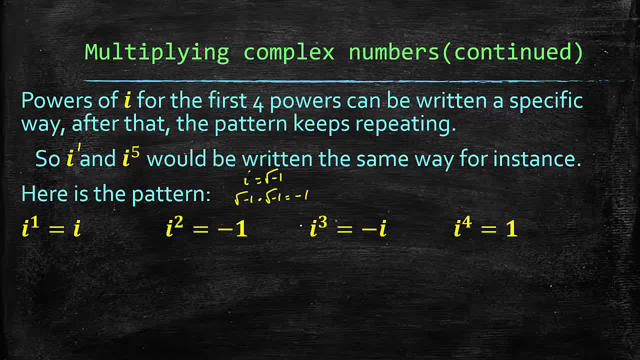 the square root. you get rid of that square root and you're left with just negative one. Okay, i to the third power is negative, i, So again same thing. You can think of this as square root of negative one times the square root of negative one. 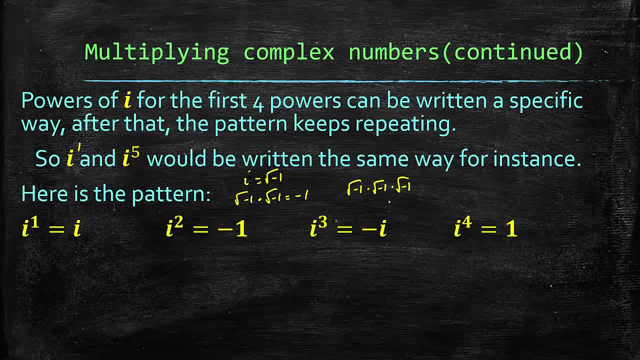 times the square root of negative one Again. so the square root symbols cancel out. so you have negative one times the square root of negative one. We don't want that because we can't have the square root, so we just write it as i and. 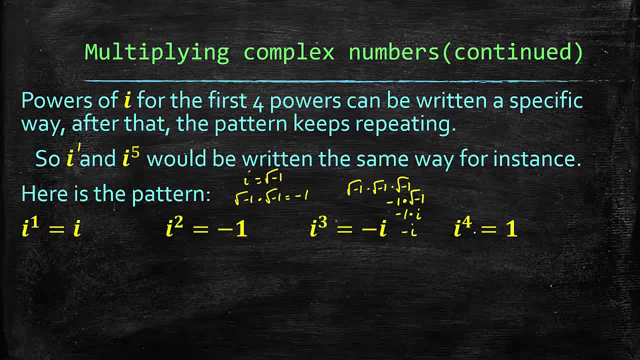 negative one times, i is negative i, and so on and so forth. Okay, So you can kind of justify how you get to here. Okay, So now that you kind of have those rules, what you do is, once you get past four and 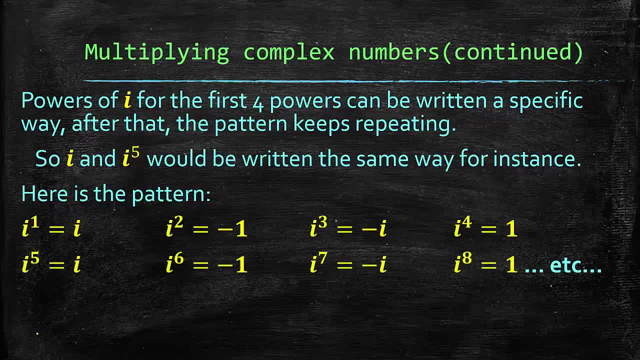 you go back over to the i to the fifth power, it repeats itself. Okay, So what you can do, there'll be a shortcut that I'll show you in a little bit that you can kind of use to figure out what i to any power is quickly. 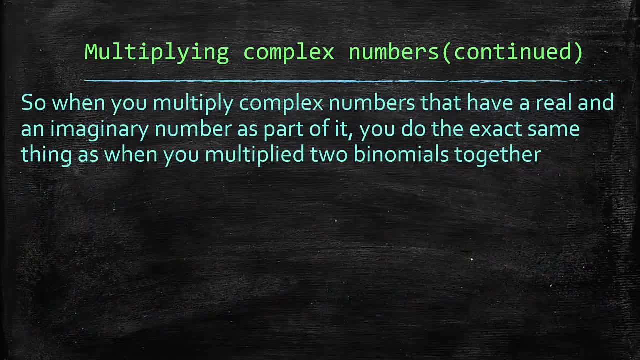 Okay. So when we multiply complex numbers that have a real and an imaginary number as part of it, you do the exact same thing as when you multiply two binomials together: You use FOIL. Yay, FOIL's back, All right. 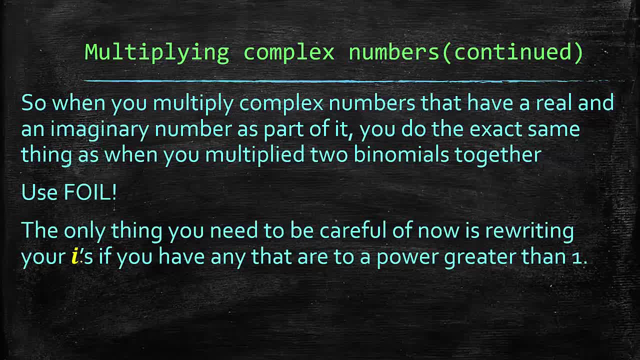 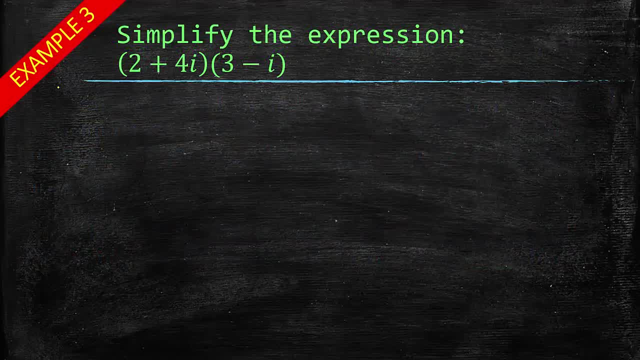 The only thing you need to be careful of is when you're rewriting anything that has an i in it, that is, to a power greater than one. you need to be aware of what we just went through. So, for example, we have two plus four. i times the quantity or times the difference. 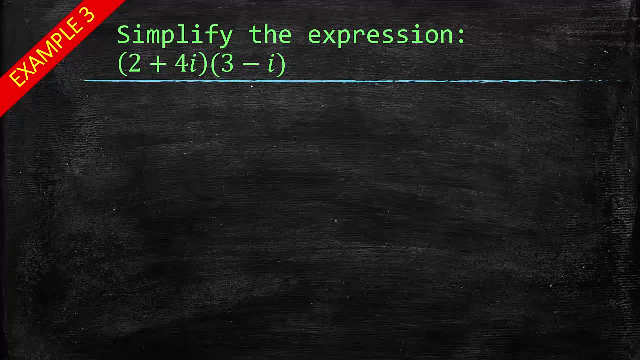 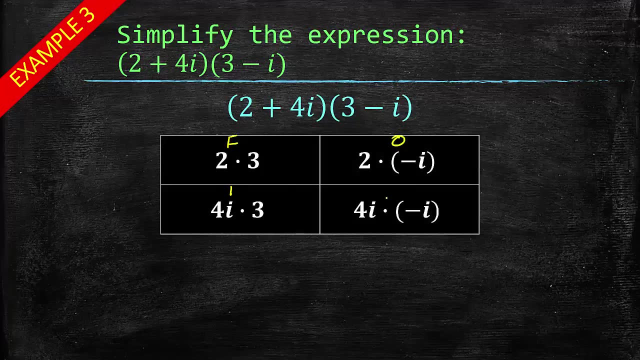 Okay, The difference of three and i. So we use FOIL. So don't forget, we have our box. Okay, First outer, inner last. All right, So we've got our first terms: two and three, Two times three. 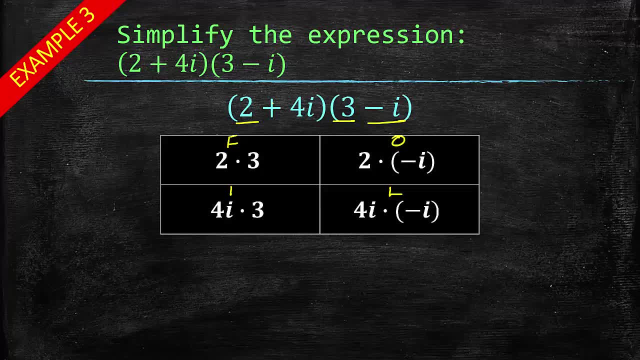 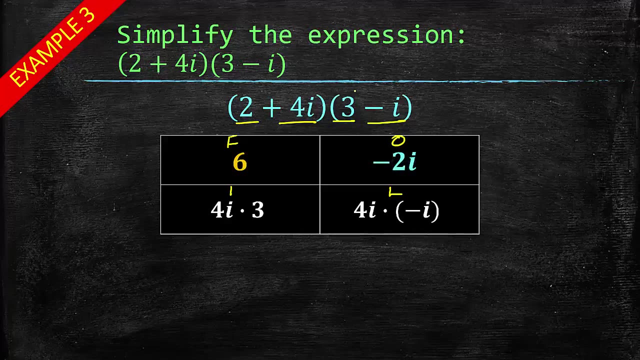 We've got our outside terms two and negative i. Then we have our inside terms four i and three. And then we have our outside terms four i and negative i. So when we multiply two times three, we get six. When we multiply two times negative i, we get negative two i. 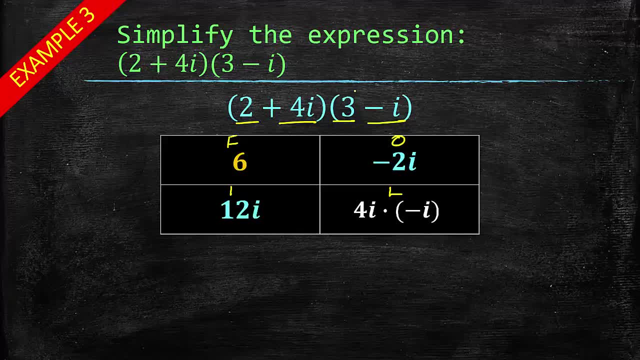 When we multiply four i times three, we get twelve i. When we multiply four i times negative i, we get negative four, i squared. This is what I said you need to be careful of, So that i squared is going to become negative one, remember. 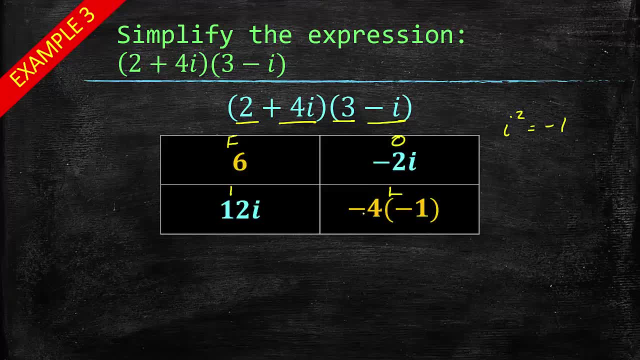 Because i squared equals negative one. So now we have negative four times negative one, Because remember it was four negative four i. Okay, This means negative four times i. So negative four times negative four is four. We add our constants. 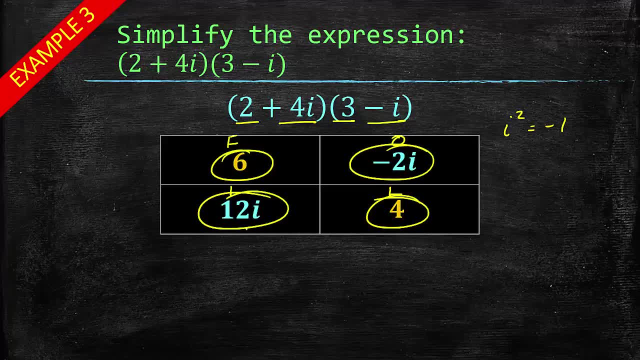 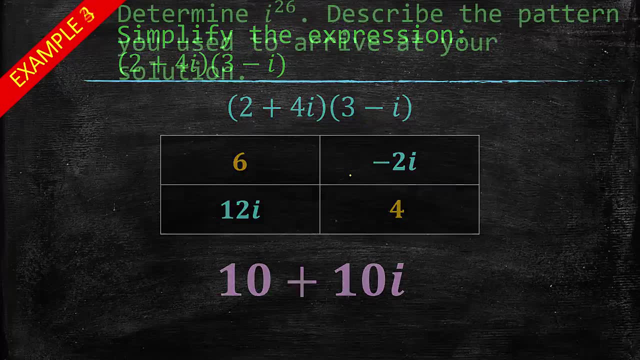 So six plus four, we add our imaginary numbers twelve, i minus two i, and we get ten. i plus ten i. We get ten plus ten i. Okay, Determine what i to the twenty-sixth power is. Describe the pattern you use to arrive at your solution. 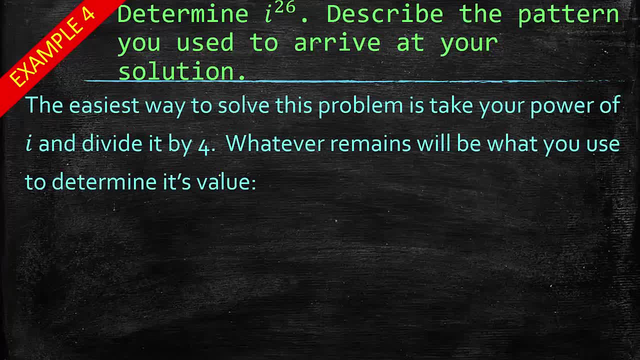 All right, Here's where I show you the shortcut. Easiest way to solve this problem is: take your power of i, So in this case twenty-six. Divide it by four. Why four? Well, if we go back, remember, we had different things for i, for i squared, for i to the. 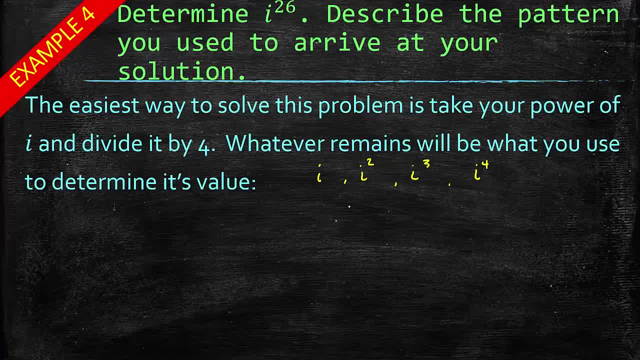 third, and then for i to the fourth. Okay, And then it repeated itself. So if we divide by four, we can keep coming back to this original thing here. Whatever's left over is what. it'll be, the same as being raised to the power. 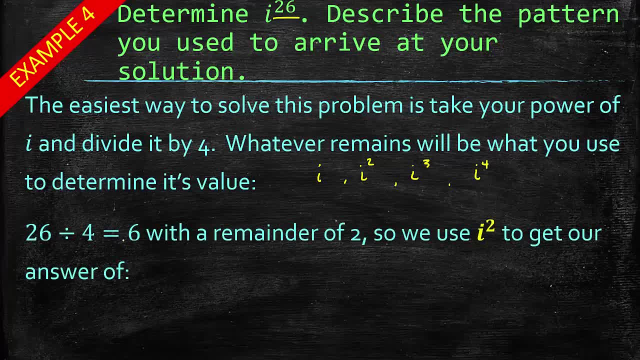 So, for example, i to the twenty-sixth. We take twenty-six, we divide it by four, which is six. that has a remainder of two. This is what we're looking for. whatever the remainder is All right. So we use i squared to get our answer, because the remainder of two becomes i squared. 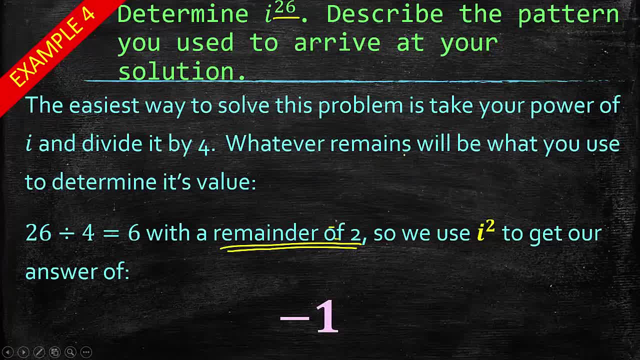 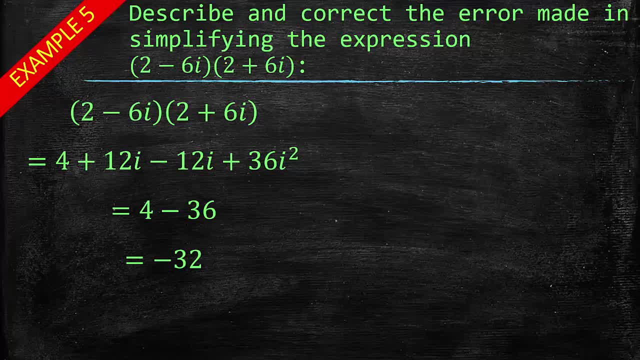 Negative one Nice and simple. Last example: Describe and correct the error made in simplifying the expression two minus six. i times the sum of two and six. i So again we use FOIL, or you remember your rules about multiplying by things that are. 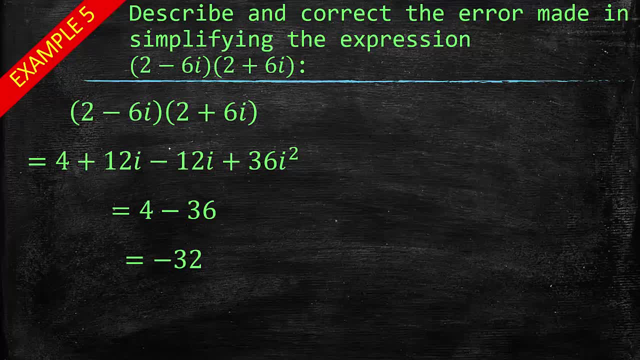 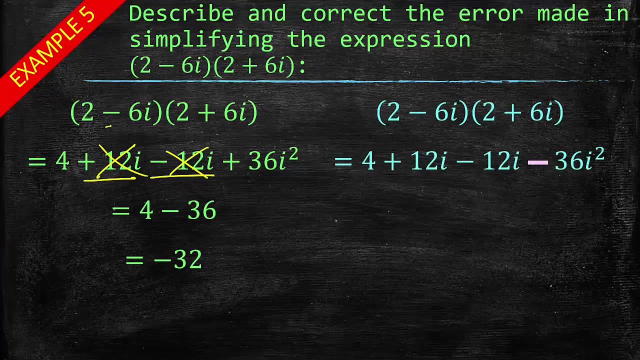 exactly the same, Except for their middle operation. So if you do, you're going to remember that this is going to cancel out the twelve i and the negative twelve i Gone Buh-bye. Okay, Here's the thing: When we do this, negative six i times positive six i is negative thirty-six i. 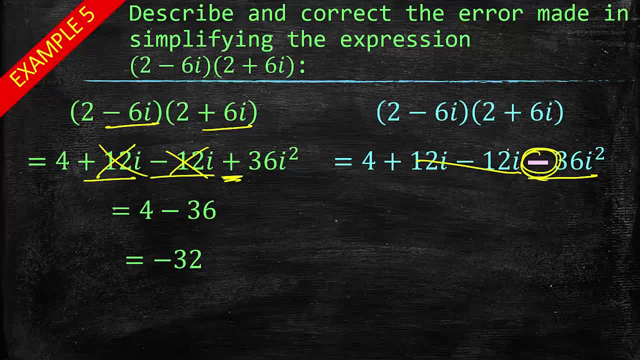 They did a positive, All right. So, yes, this will still cancel out, but that changes the whole problem when you carry it all the way through, See, because this becomes four plus thirty-six and you might be trying to figure out how. 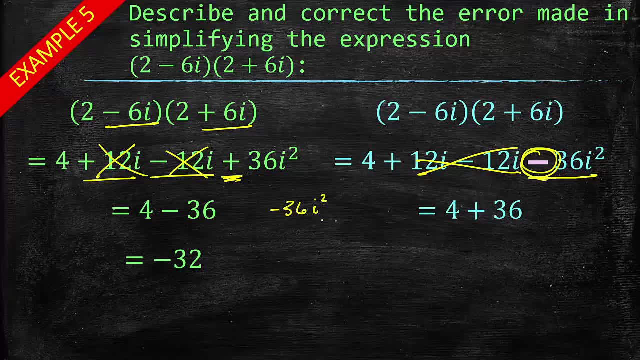 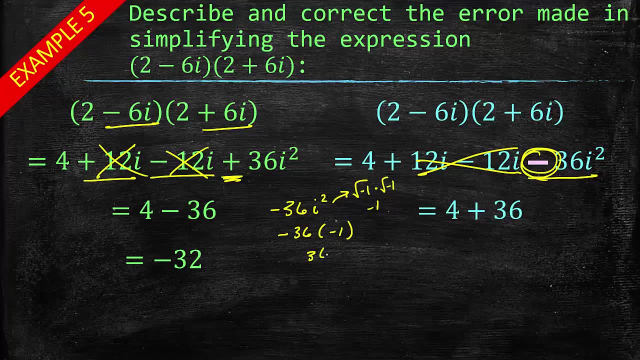 We take negative thirty-six times. i squared. i squared, remember, is the square of negative one times the square of negative one, which is just negative one. So i squared is negative one, So negative thirty-six times negative one is a positive thirty-six. 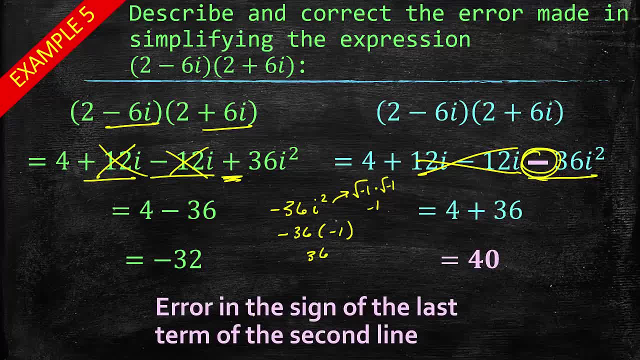 So that gives you forty. So the error was in the sign of the last term, of the second term, So that gives you forty. All right, So that's the second line And that's all there is to it. So if you can just go back and memorize, like the i to the first, second, third and fourth, 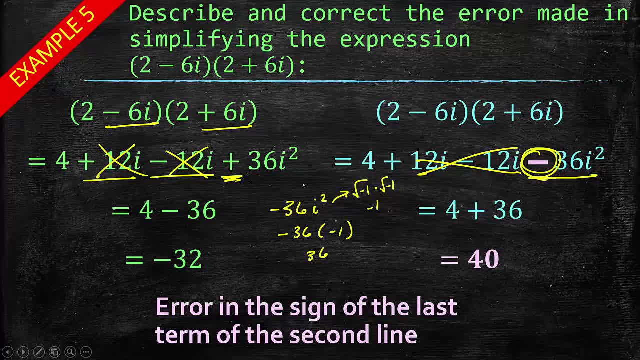 power and then just remember the quick way of doing it. you should have no problems. I mean really, other than that the rest of it's all stuff that you've done before. So that's all I got for you. You guys have a lovely day. Ask if you have any questions.